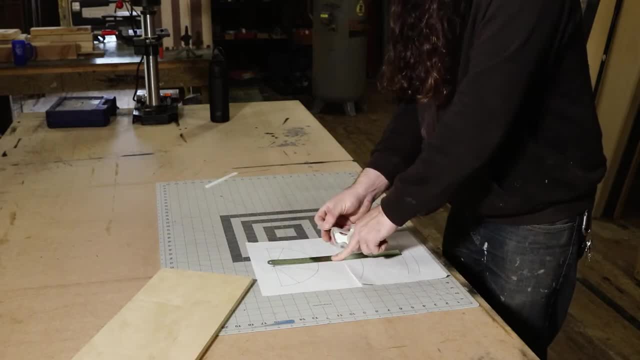 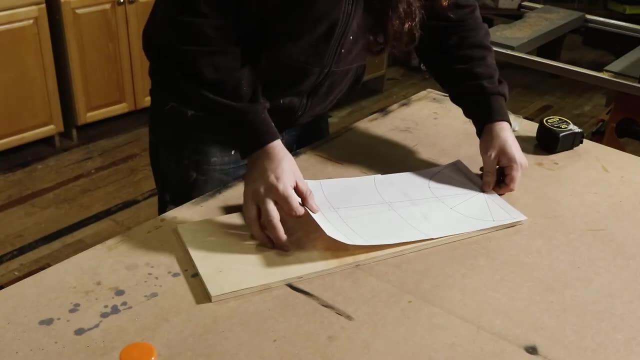 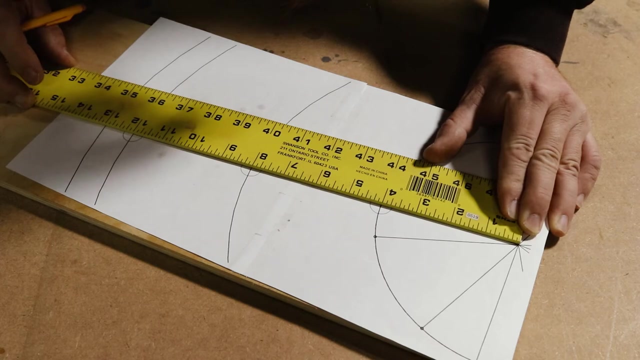 was made to fit on a piece of legal size paper, which I didn't have on hand, But Adobe Acrobat allows you to print out large designs on regular 8.5x11 paper by choosing the poster option. When Games Maker designed this jig, he was also using a separate jig to cut out the diameter of 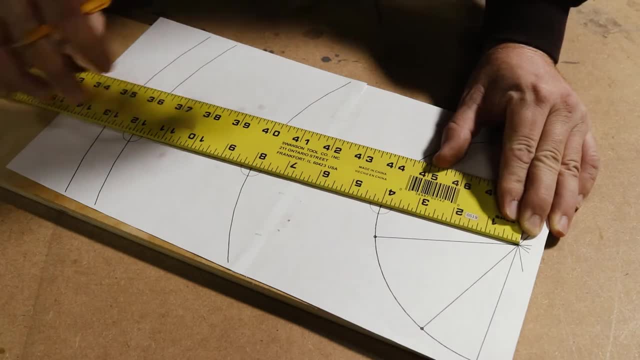 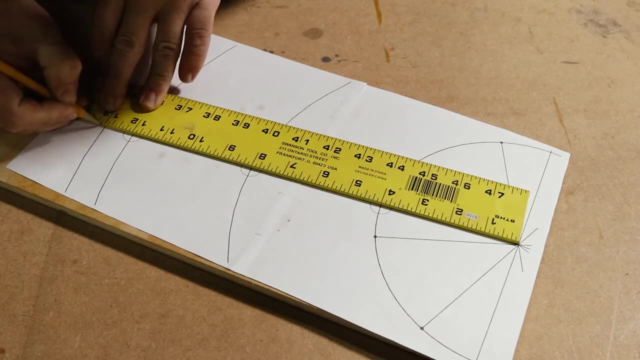 the game board as well as the base. But since I'm doing an octagon base, I figured I could just add one more location to this jig, so I could use it to cut out the game board as well. So here I'm just adding a mark at 13 and an eighth from center, because I've got a lot of ink in here. I could just cut out the small parts of the board, And this jig is really easy to use. I've got a lot of ink in here. I've got a lot of ink in here, And I've got a lot of ink in here, And I've got a lot of ink in here. 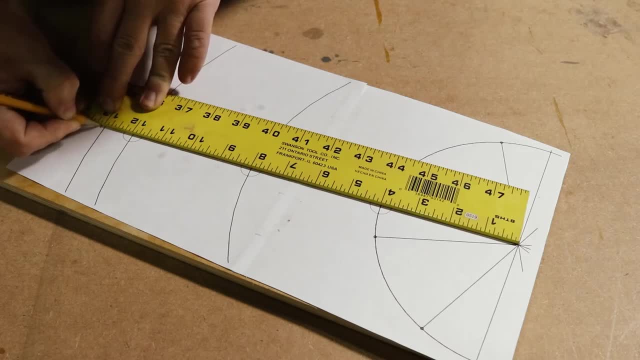 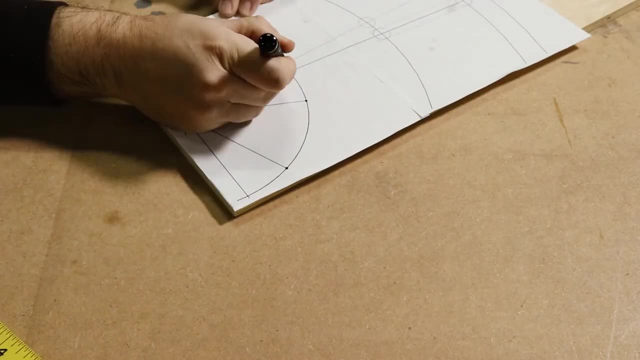 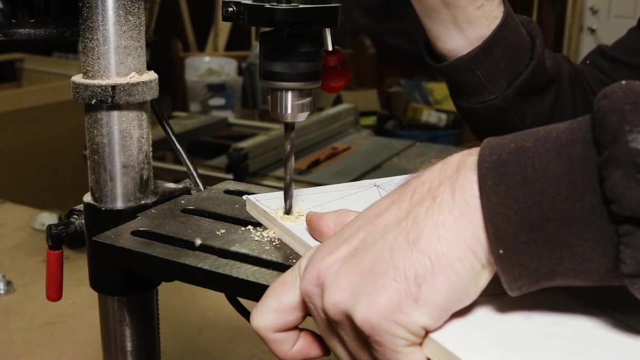 from center, because I'll be using a quarter inch router bit to cut this. so this will give me a board with a diameter of exactly 26 inches. For the peg locations, I'm using a 5- 16th inch drill because I happen to have these. 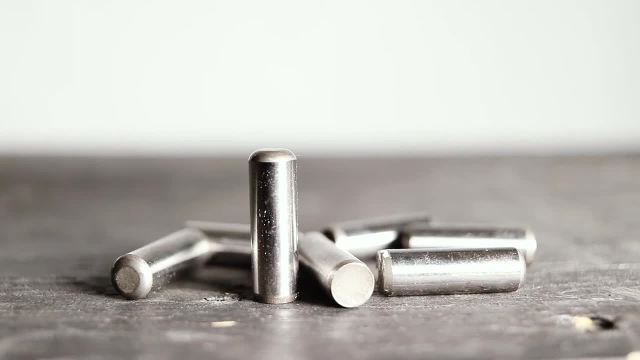 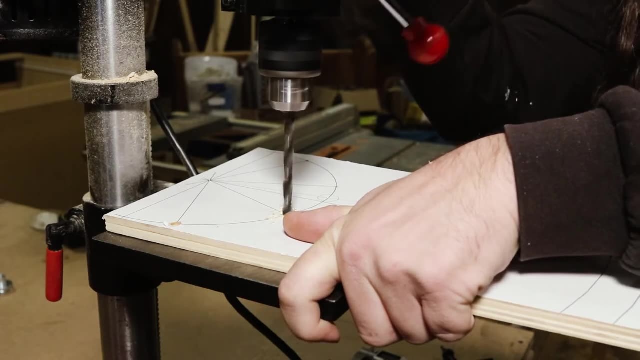 steel location pins from my machine shop that I thought would look really cool. So usually you'll see these boards with either brass or wood or sometimes rubber pins in the center, but again I had these on hand and I think they look really nice. 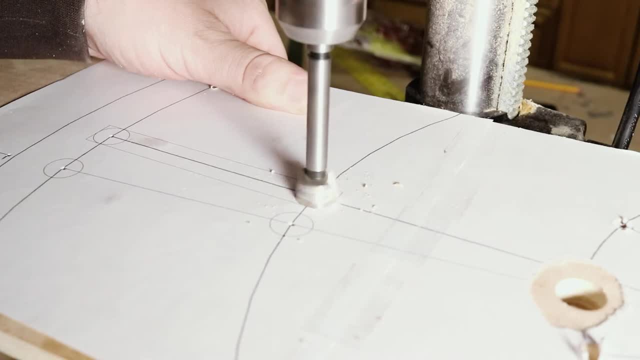 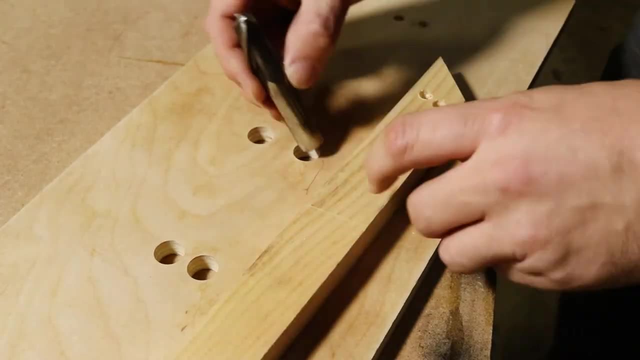 And for the larger holes, I'm using a 5- 8th inch Forstner bit, since I'll be using a 5- 8th inch guide bushing on my router. Now. these two holes here need to be connected and routed out, so I'm making some rough lines. 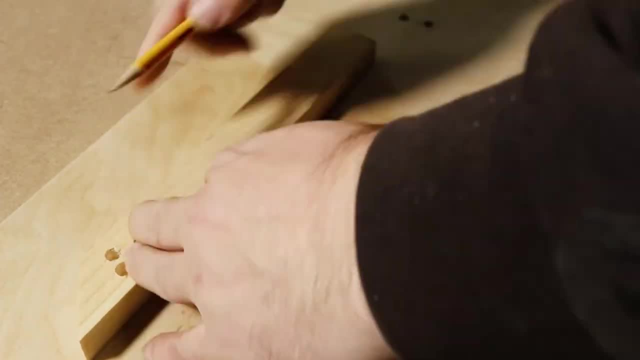 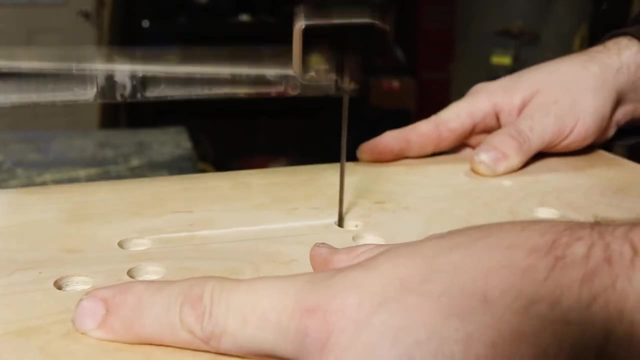 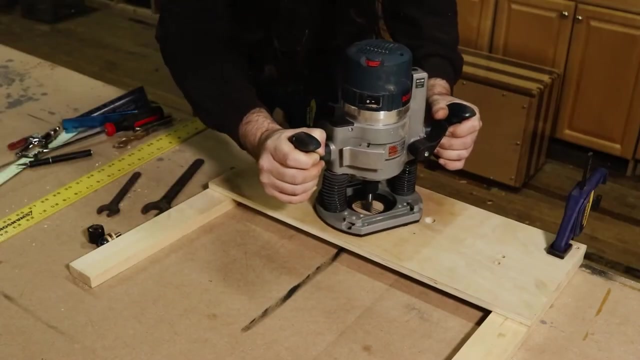 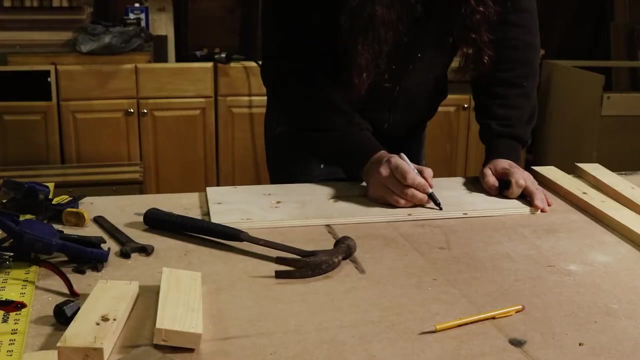 between them. This section of the jig is used to make the intersecting lines that divide up the four quadrants of the board, And I'm using the scroll saw to get close to the line, but not super close, because I'm going to use a router to make that perfect. 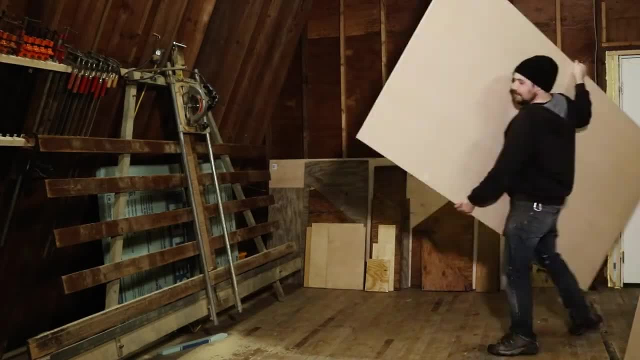 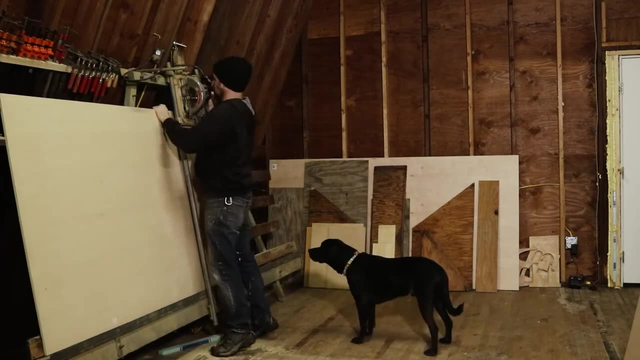 And now it's time to start cutting the plywood. I'm using half inch plywood and I cut it down to around 27 inches wide, which would give me a little bit of play on either side. I'm cutting out the circle. If you're using the method that GamesMaker uses, you can actually get four game boards. 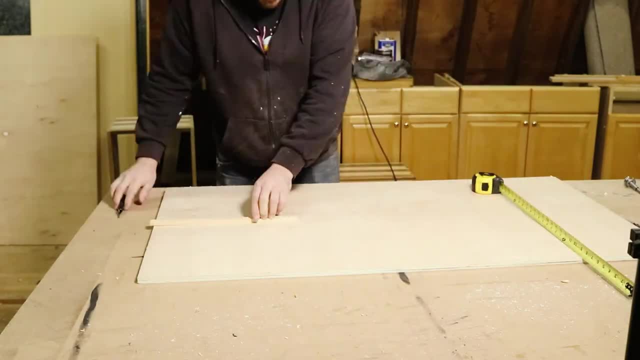 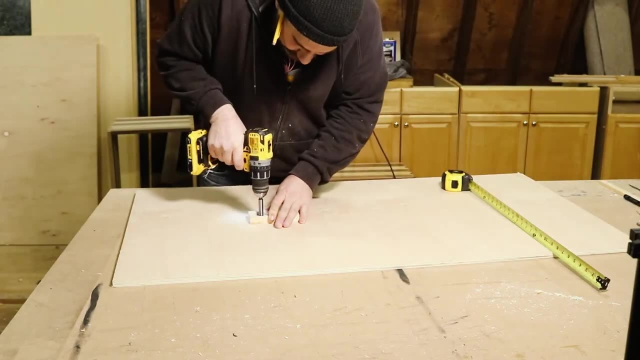 and bases out of one sheet of plywood, But in my case, since I'm doing an octagon base, I had a little bit more waste, but I was still able to build two boards and I had some plywood left over. In Crokinole, your main goal is to get your pieces into a small hole at the center of 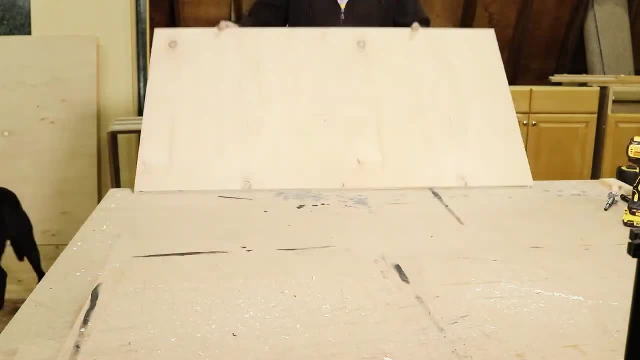 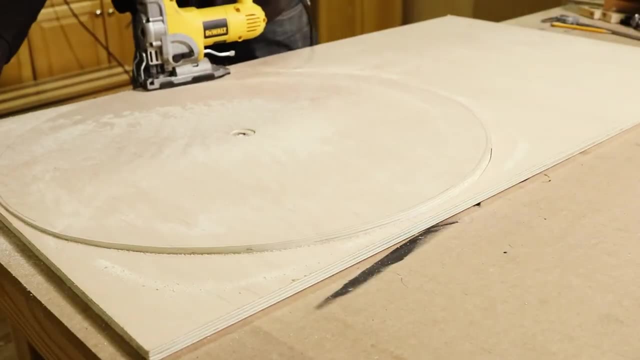 the board, which is an inch and three eighths wide. So here I'm using a Forstner bit to get that started, as well as drilling a 5- 16th inch hole through the board all the way, Which I'll use with my locating pin to align my jigs later. 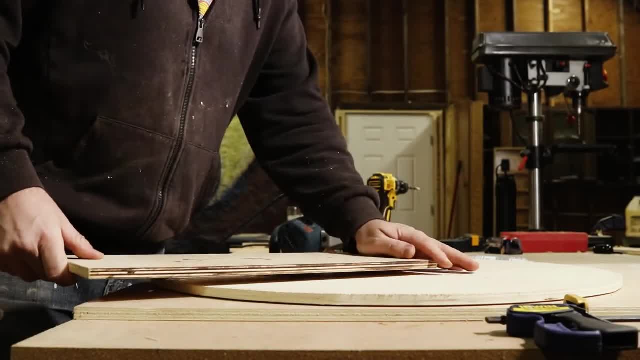 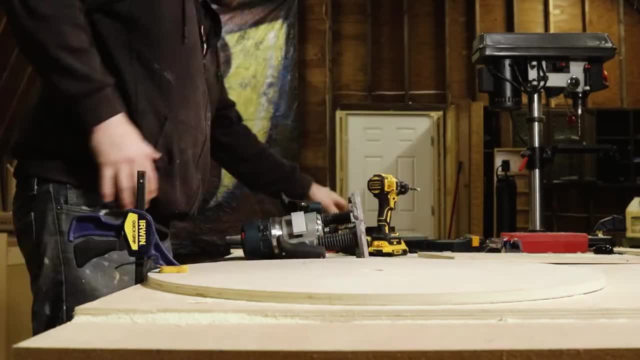 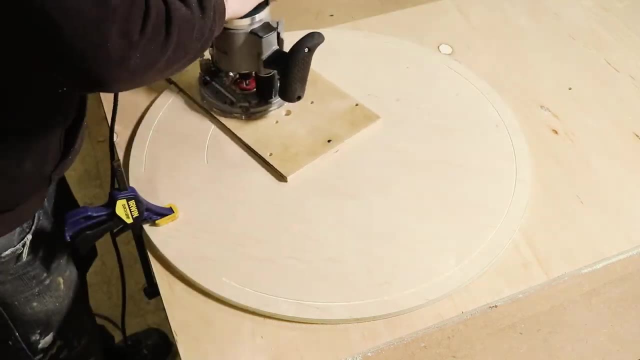 And now we finally get to start using the jig that we built earlier. So I use the center locating pin to align everything and, taking my time and doing multiple passes, I get the board to its final 26 inch diameter. Next I put an eighth inch bit in my router and started cutting the concentric circles. 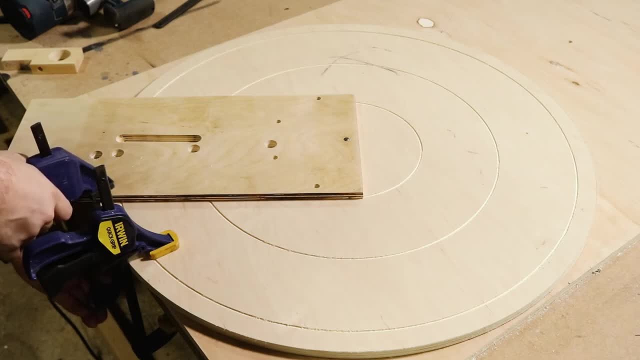 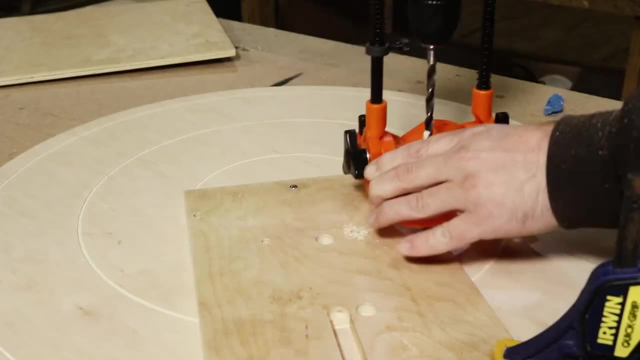 Once all the concentric circles were cut out, I could switch over to drilling the holes for the pegs, as well as cutting the intersecting lines that make up the four quadrants, And the beauty of this jig is that you drill your first four holes, which I'm drilling. 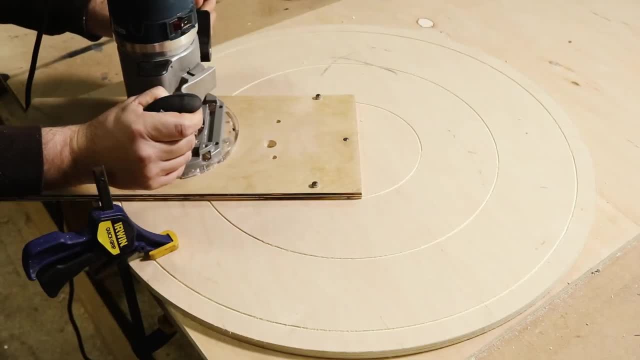 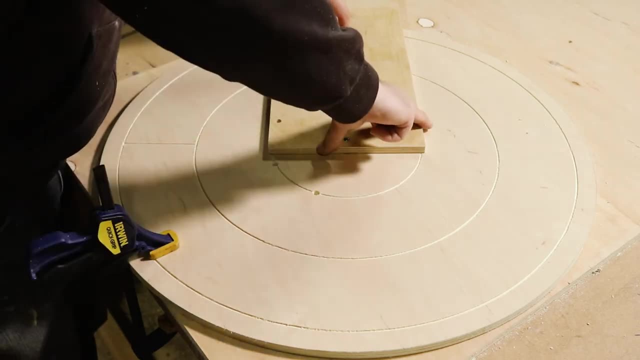 about a quarter of an inch into the board. Then you use your router to cut the first line. Then you rotate the jig 90 degrees, which is super easy because you can just use the last two holes you drilled to align it with your pegs. 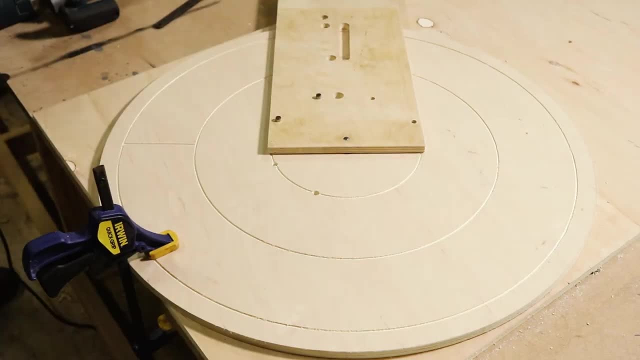 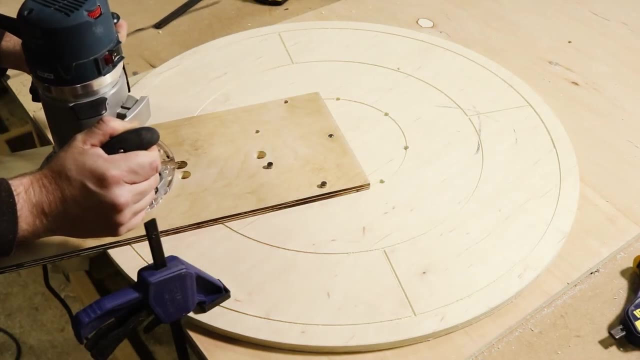 Now, with the jig in this alignment, you drill your next two holes and cut the intersecting line And you just repeat this two more times, using the previous holes drilled to align your jig at 90 degree intervals And once you're done, you have all eight peg holes drilled and all four quadrant lines. 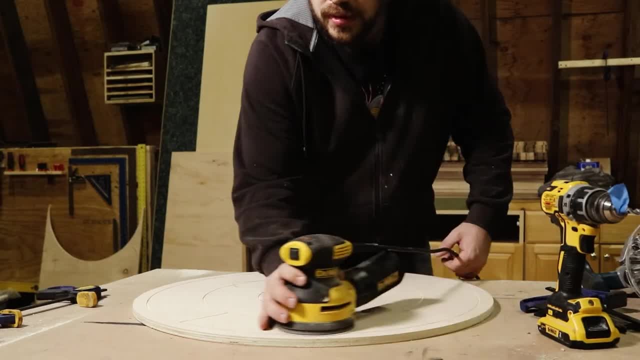 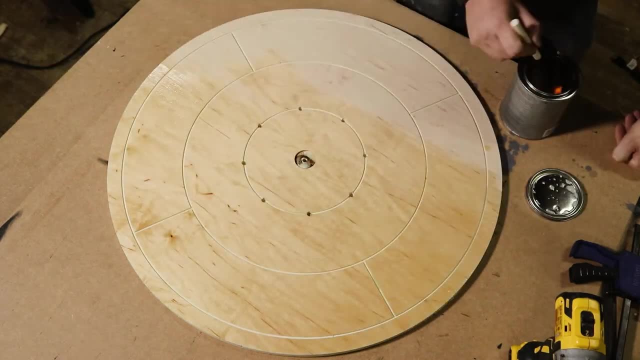 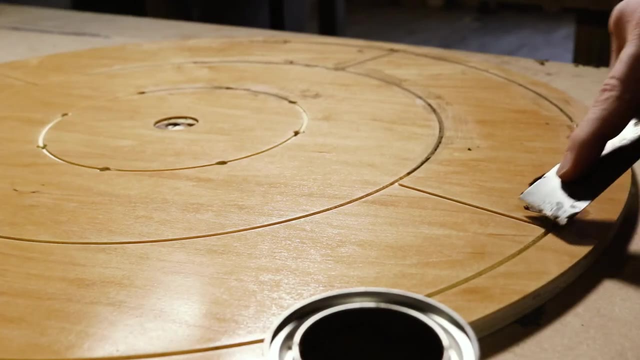 cut in perfect alignment. At first I thought I was going to fill the lines in with some epoxy that I had, But in the end I just went with some walnut wood filler. I did give this two coats of filler and I sanded in between each coat. 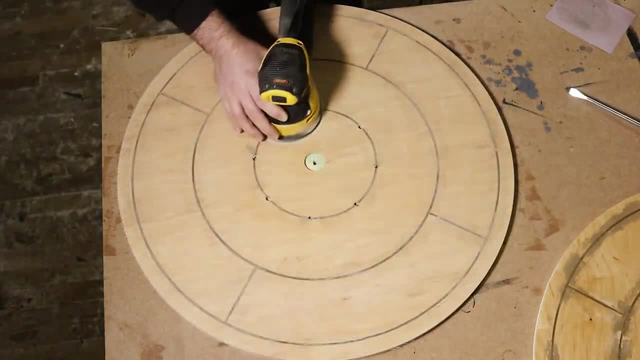 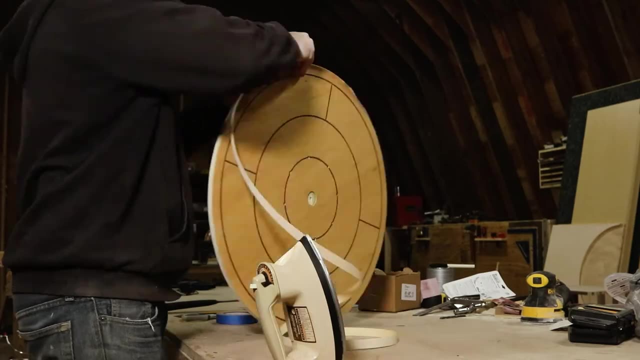 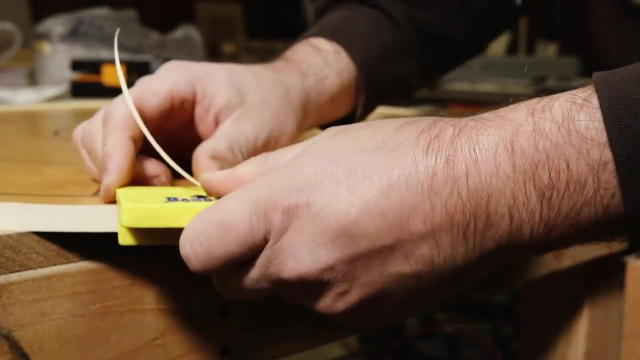 And then I did one final sanding on the whole board to make sure everything was nice and flat. I ran some edge banding around the boards and originally I thought I wanted both of these to have a dark edge banding to match the concentric circles. 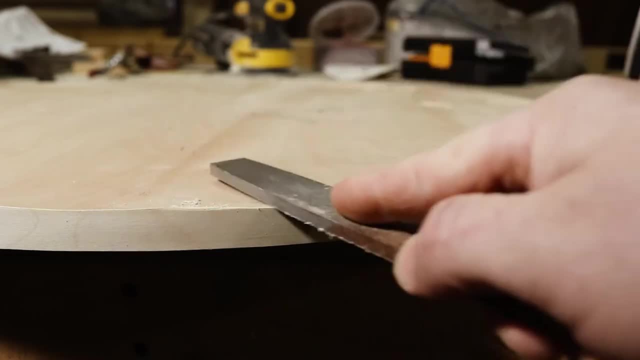 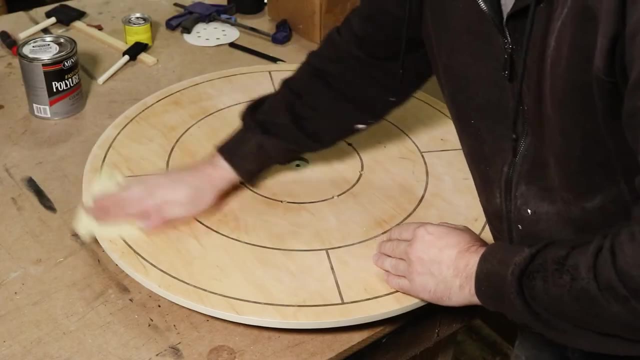 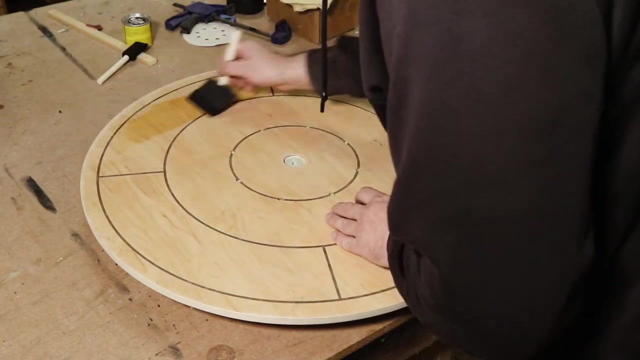 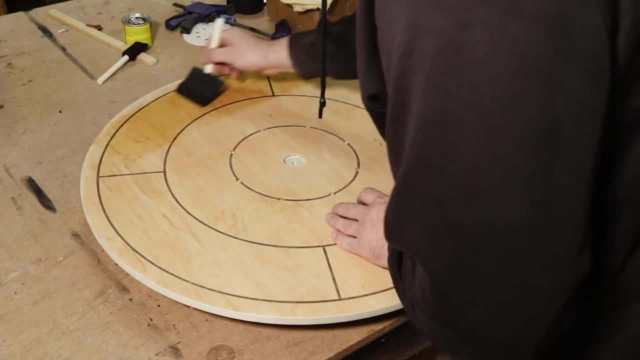 on them And I started applying the final few coats of polyurethane. I think I ended up doing a total of three more coats on each board, scuffing them up in-between each coat just to make sure I had a nice flat glassy surface. 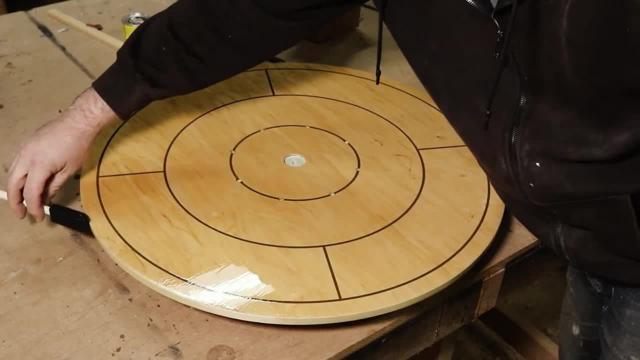 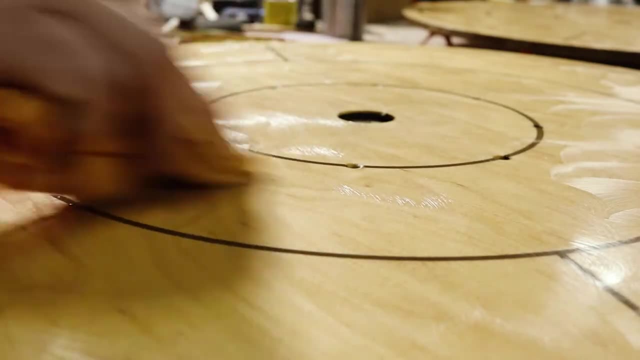 So between the two boards, this ended up being a couple days of applying the poly, letting it dry, scuffing, applying another coat over and over again until I was happy with the finish. Okay, super excited to try out the game, I gave one of the boards a quick coat of wax and cut a dowel. 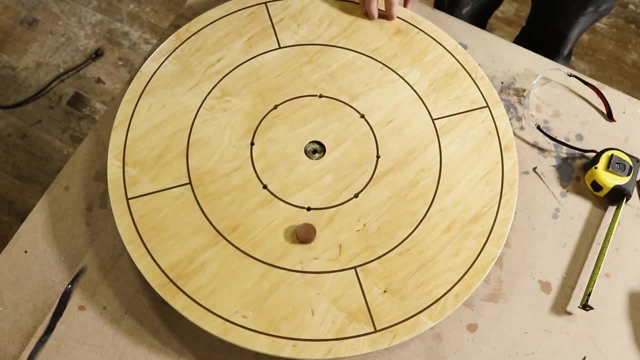 to make a temporary game piece and I wasn't very good at it. As an aside, the discs were the one thing I did end up ordering online, because I had zero desire in making about 50 of these things by hand and they're really cheap online, So I'll put a link for where I bought these in the 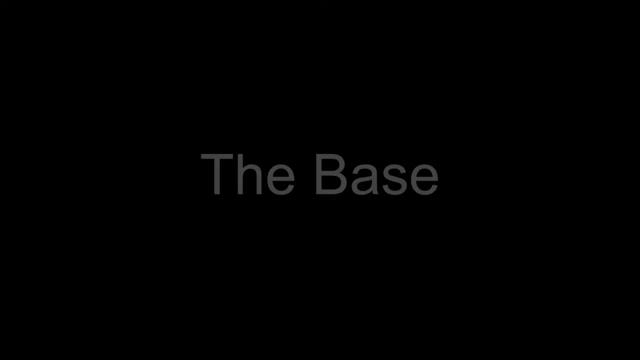 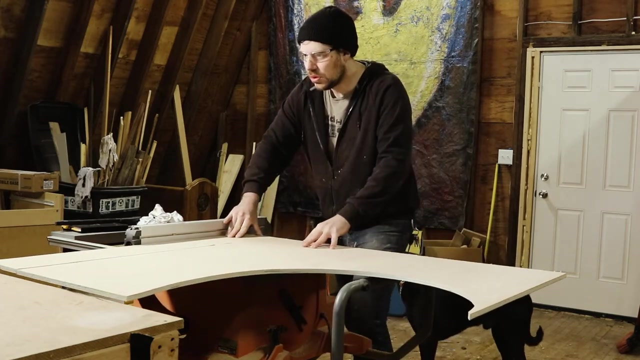 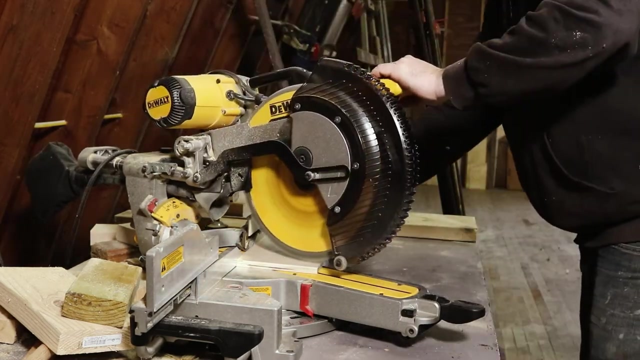 description below. And now it's time to make the base. So I grabbed some of the leftover plywood and I cut these into six inch wide strips. Then I took it over to the miter saw, set my angle for 22 and a half degrees, made my first cut and then I measured 12 and three quarters on the long edge. 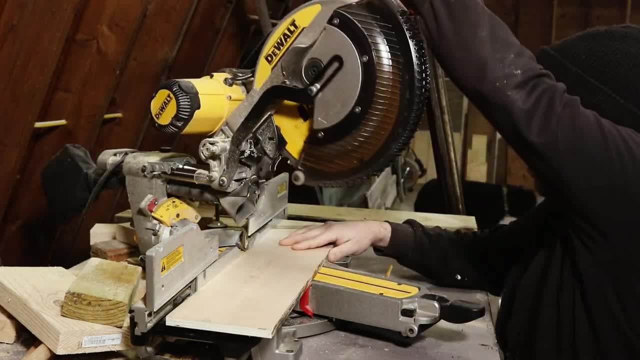 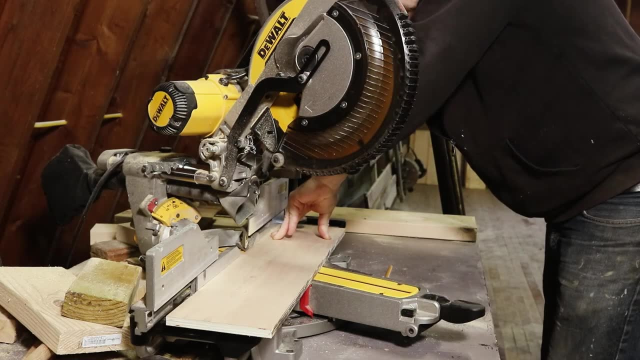 and set a stop block. Now I just used the measurements that Tyson over at the Geek Woodshop channel was using, and I didn't take into account that he used thicker rails on his board and he could cut a rabbit into them, So the ditch on my board ended up being a little bit. 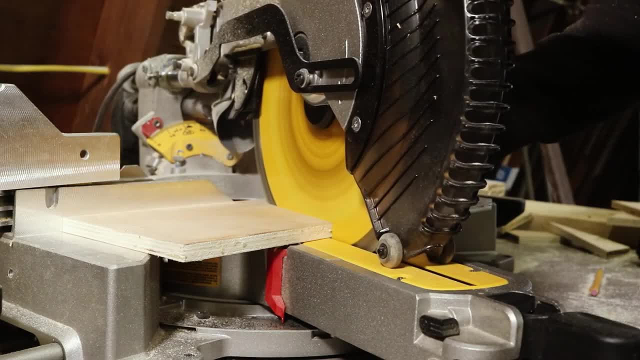 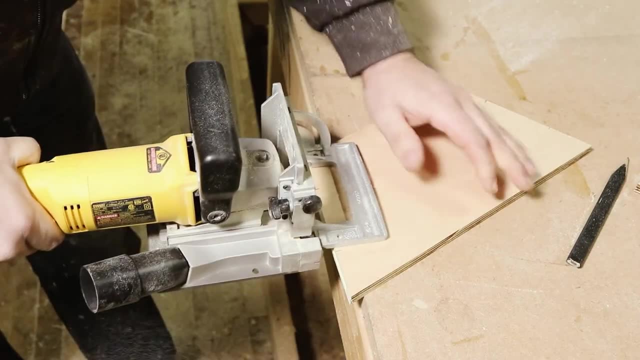 wider than it needed to be. So in the future I would alter these dimensions a little bit and make them a little bit shorter. And now I'm ready to put all the pieces together. So I grabbed my biscuit joiner and made some slots, just to help with alignment and to keep things a little. 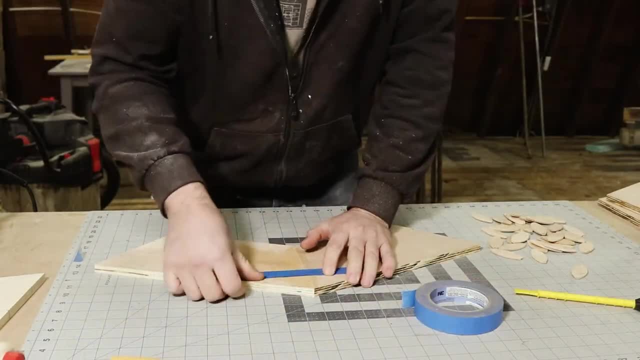 bit snug while doing the glue up And I just used some painter's tape to keep things together while the glue dried. Once I had all the pieces glued together, I took a little bit of tape and I put it on the side of the board and I put it on. 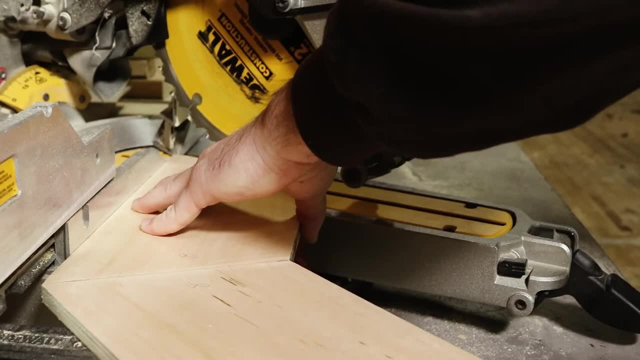 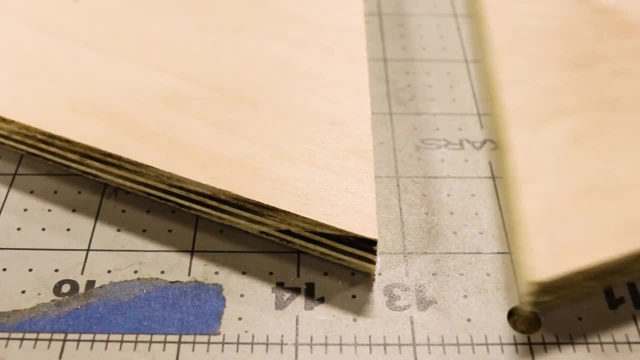 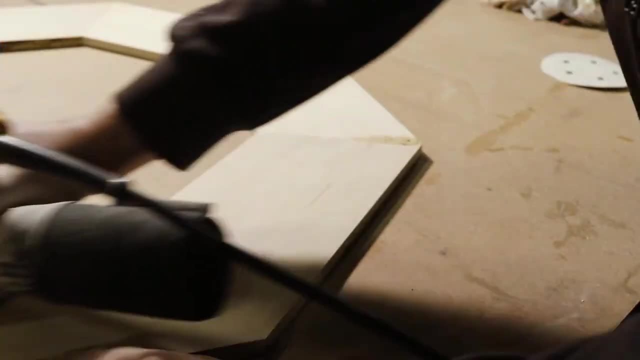 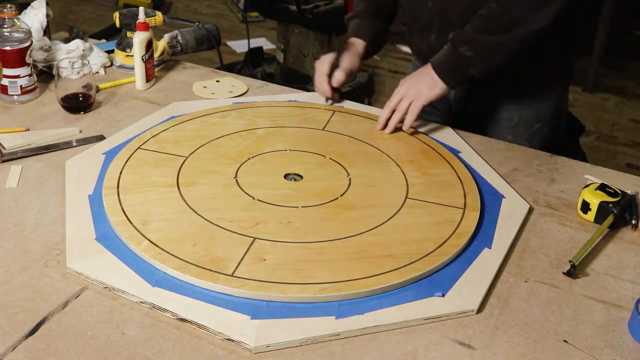 because there were so many cuts made on this, So it just was a matter of taking it over to the miter saw and making little tiny cuts until everything lined up perfectly. Next I put some painter's tape on the base and used this jig to line the top up over the base. 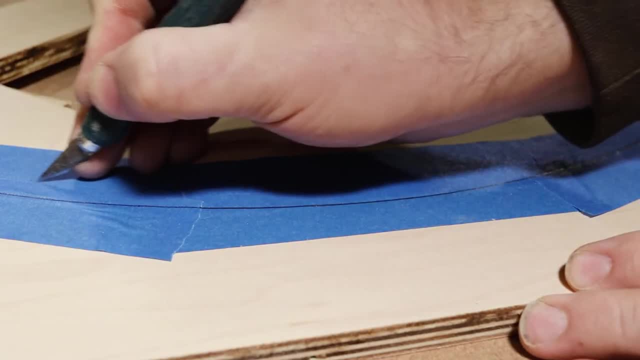 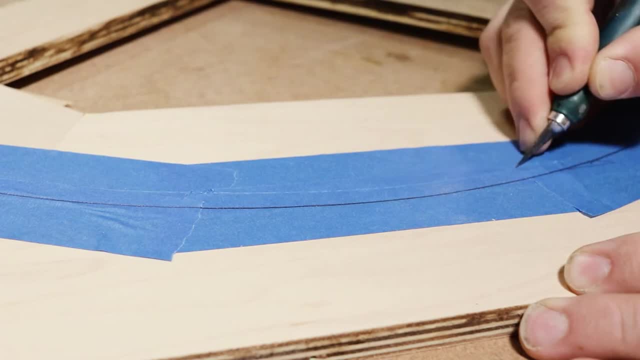 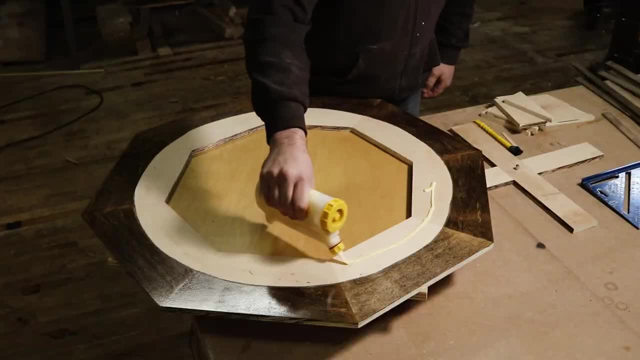 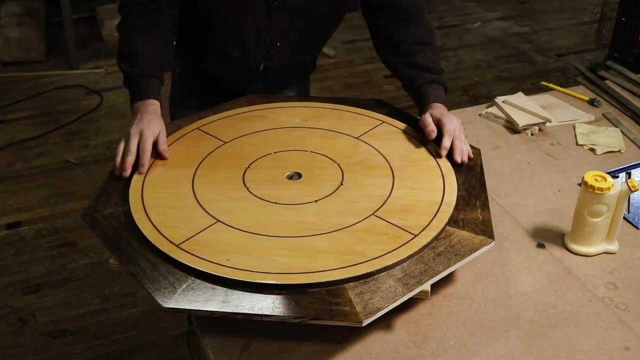 And now it's time to glue up the base. so I grabbed a bunch of clamps, put some glue on the base, used my alignment jig to get things pretty close to center and then just used my tape to double-check everything and got everything squared up and put all my clamps on. 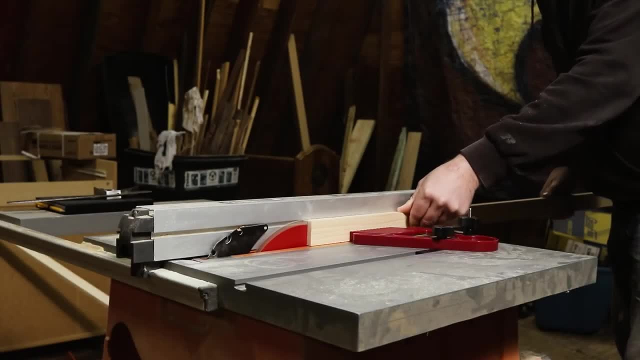 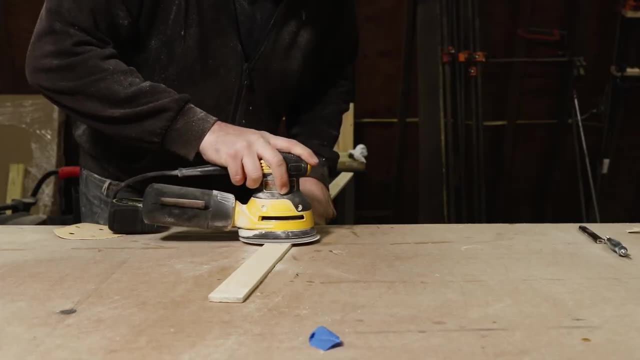 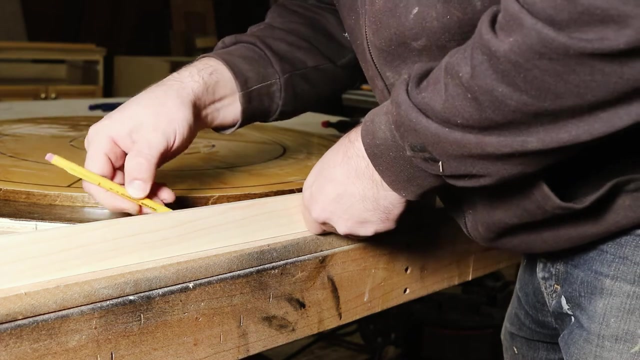 And the last little bit we have to do is make the rails that go around the outside of the base. So I grabbed some inch and a half stock and ripped it down to quarter inch wide and gave it a quick sanding set up. my miter saw for another 22 and a half degree angle, made my first cut, lined it up on the board and made a pencil mark where I needed to make my second cut. 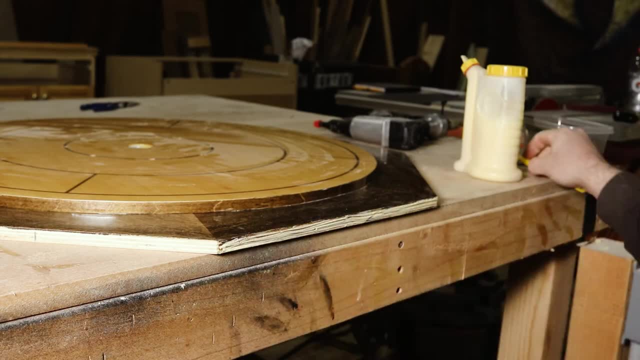 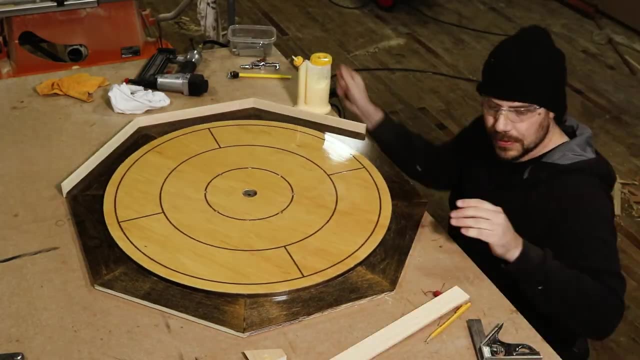 Then I just repeated this all the way around the board until I had the rail completed. This is my final cut and it's an easy one. I'm almost done with it, But anyway, I hope you enjoyed this video. I appreciate you watching and I'll see you in the next one. 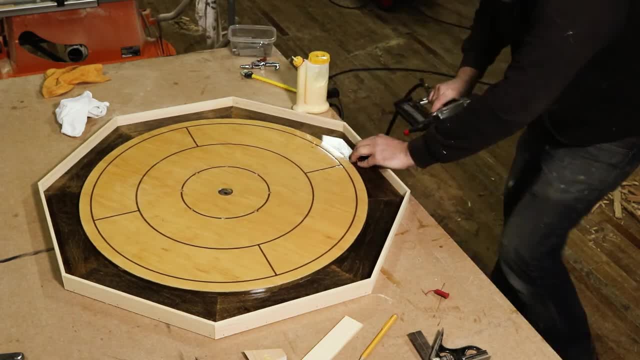 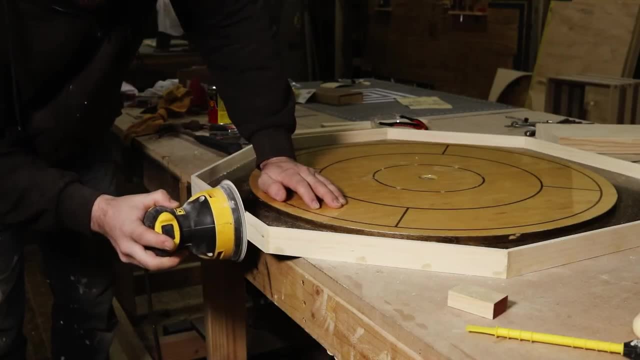 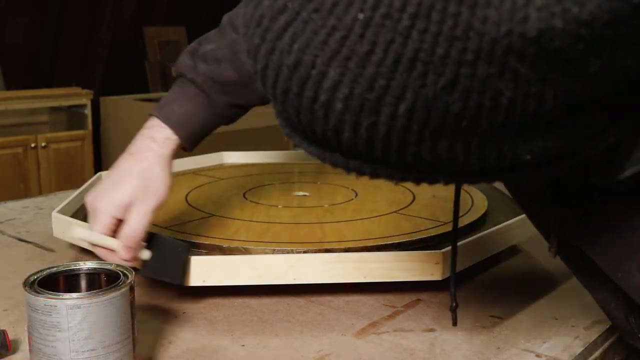 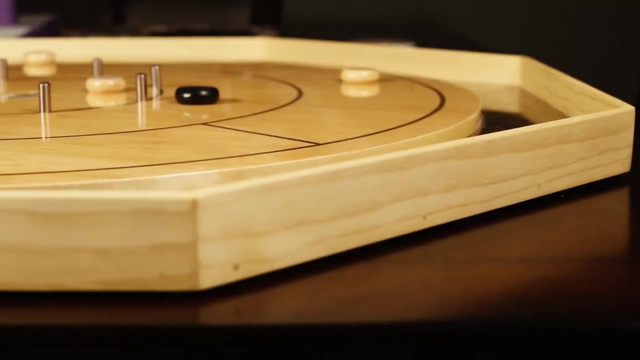 I hope you enjoyed this video. One final clean with a tack cloth and two more coats of polyurethane on the rails and the board is done. I am really happy with the way these came out. They were a ton of fun to build. 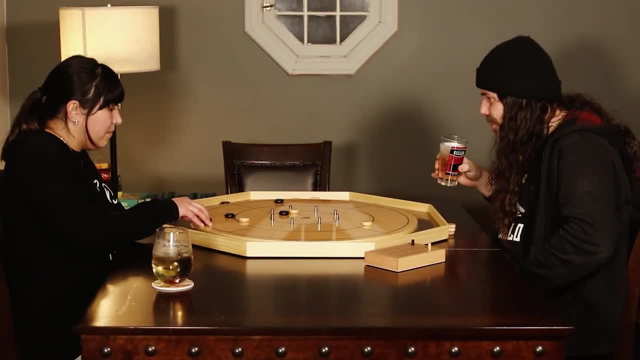 And they came at $1,000.. That's a lot. That's a ton of fun. to build is even more fun to play. My girlfriend and I have been playing a ton over the last week and I gotta say it is a really, really fun game. 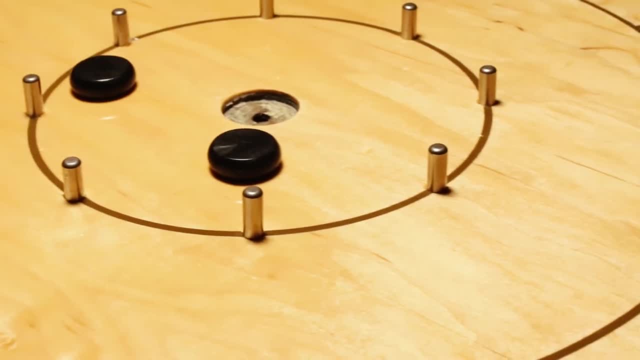 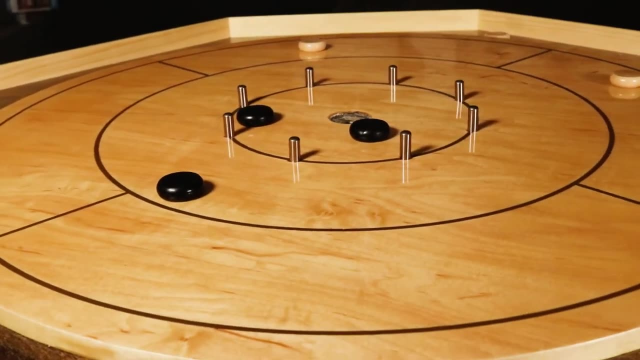 It's super easy to learn and, while it's obvious that you could get very skilled at it, even at our novice level, I didn't feel frustrated or angry at a bad move that I made or anything like that, And in fact I did find myself getting excited.